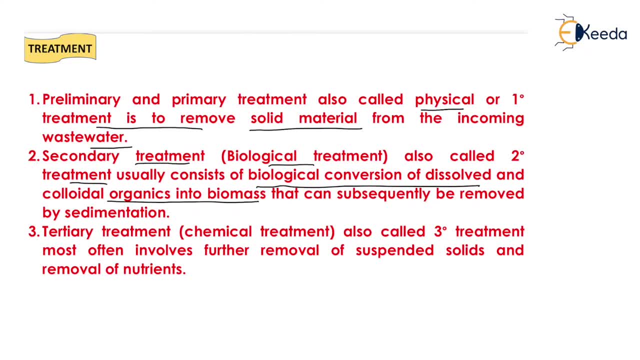 Clear Now. the next process, Or the next treatment process, will be tertiary treatment, also known as chemical treatment, also called as three degree treatment Most often involves further removal of suspended solids and the removal of nutrients from the water. But we never go for that tertiary treatment. 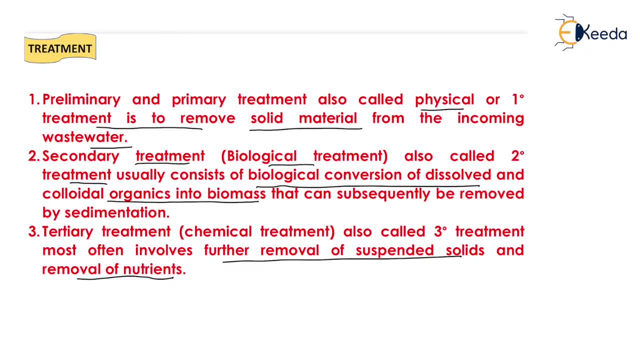 because tertiary treatment is generally required when we want to use that waste water for the drinking purpose. But in India we don't go for the drinking water or we don't want to treat the wastewater for the drinking purpose. that's why we never go for the tertiary treatment. 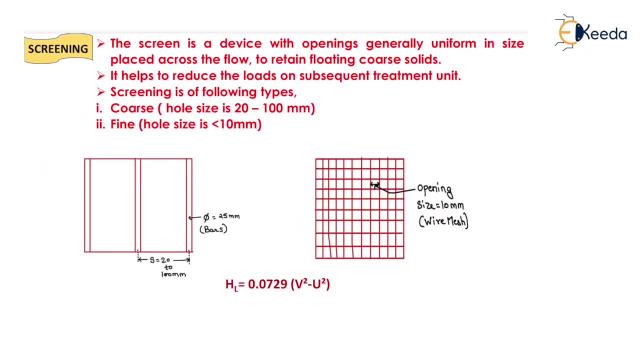 clear to all now. the first method in the primary or preliminary treatment is screening. we had already discussed that screening in the drinking water treatment process and the same screening will be there also. okay, now the screen is a device with openings, generally uniform in size, placed across the floor to retain floating coarse solids. okay, why we are using the screen? because 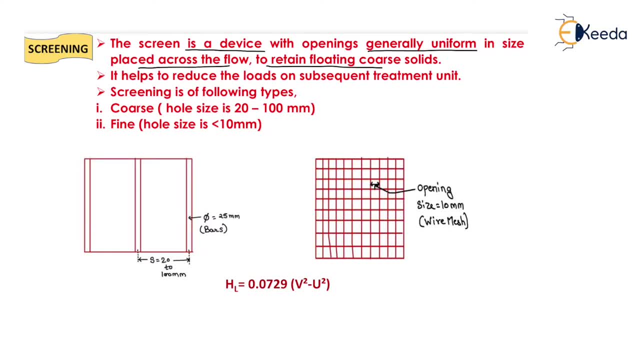 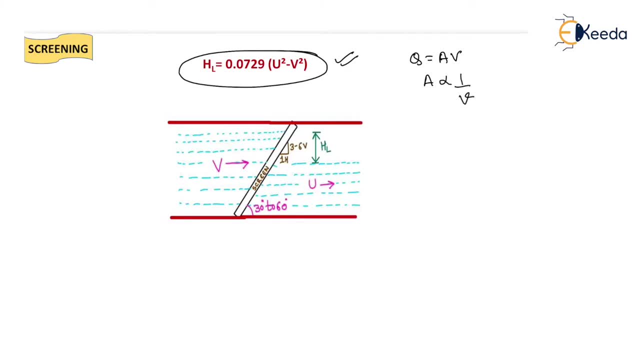 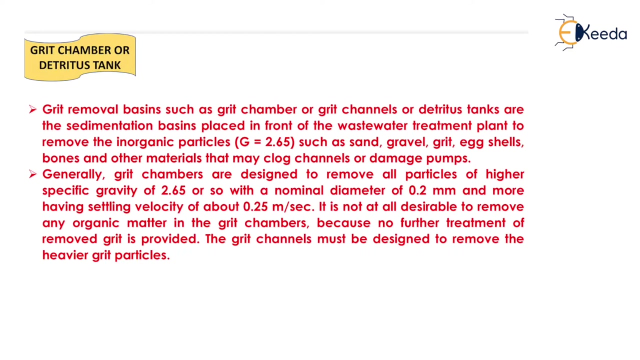 the process of the treatment process and it will help in the process of the treatment process and it will help in the process of the treatment process and it will help in now. the next process will be the grid chamber or detritus tank. now, grid removal basis, such as grid chamber or grid channels or detritus tanks, are the 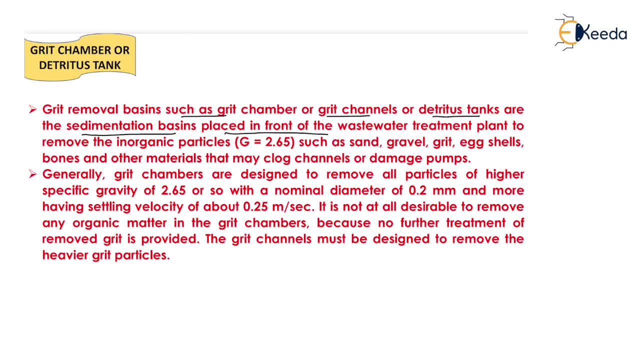 sedimentation basins placed in front of the wastewater treatment plant to remove the inorganic particle. why we want to use the grid chamber to remove the inorganic particles whose specific gravity is 2.65, such as sand, gravel, grit, eggshells, bones and other materials that make locked channels or damage pumps. 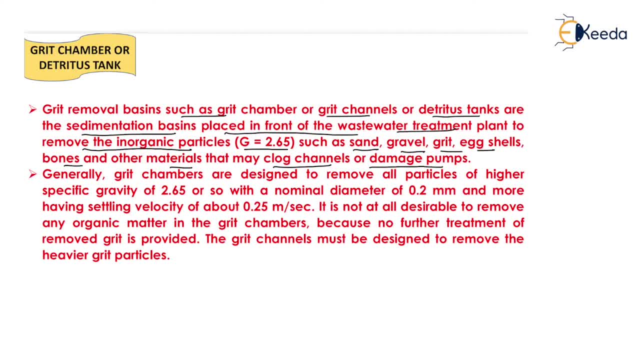 that's why we will use the grid chamber or detritus tank now. generally, grid chambers are designed to remove all particles of higher specific gravity of 2.65 or so. it means that grid chamber is generally used to remove the higher specific gravity particle, that is two. 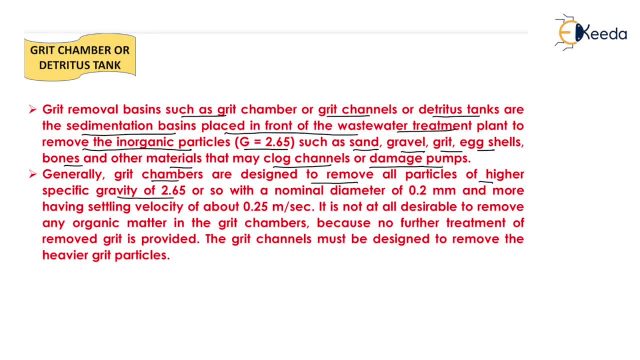 point six, five or greater, with a nominal diameter of 0.2 mm and more, having the size 0.2 mm or more, having settling velocity of about zero point two, five meter per second. it means that the velocity in the grid chamber is generally kept as 0.25 meter per second. now it is not at all desirable to remove. 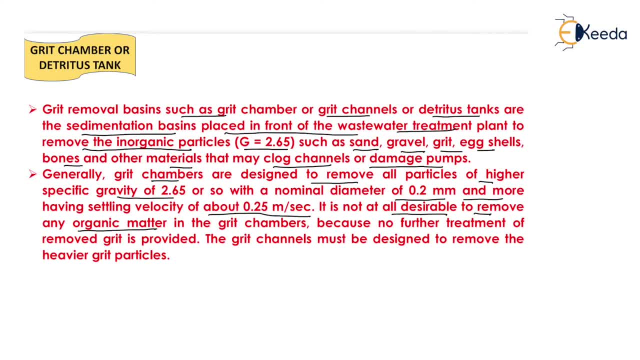 any organic matter. okay, any organic matter in the grit chamber, because no further treatment of removed grit is provided. that's why we don't want the removal of any type of organic matter, otherwise it will pollute the environment when we directly throw the grits and all the waste. 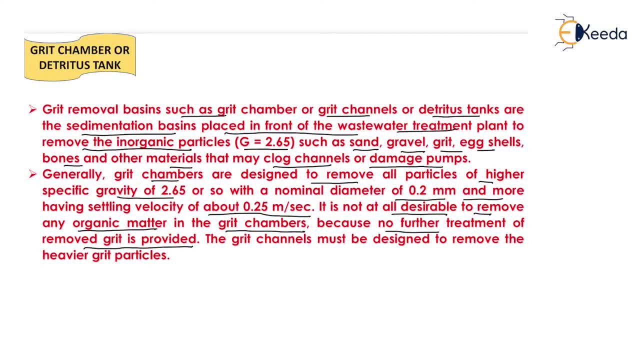 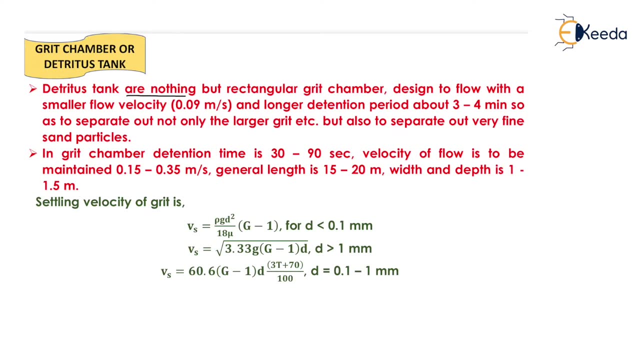 from the grit chamber into the atmosphere or into the environment. clear now. the grit channels must be designed to remove the heavier grit particles only clear now. detritus tanks are nothing. we have discussed the grit chamber. now we will discuss the detritus tank. detritus tank are nothing but rectangular grit chamber designed to flow with a smaller 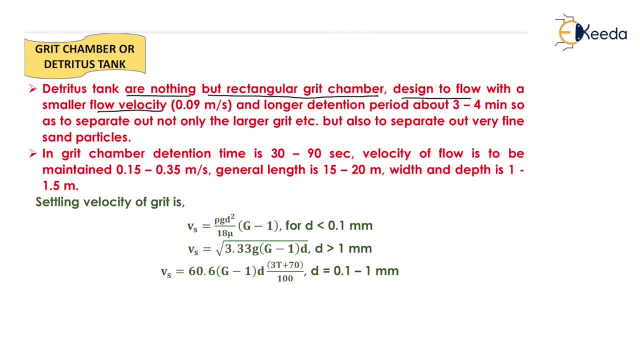 flow velocity. here we want the removal of particle on larger basis as compared to grit chamber. so we have to remove the heavier grit particles only clear now detritus tanks are nothing but rectangular grit chamber. that's why we will keep the velocity on a lower side. 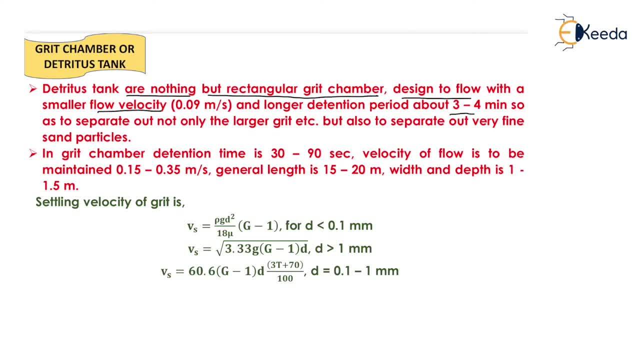 with a longer detention period of about three to four minute, and the velocity will be equals to 0.09 meter per second, so as to separate out not only the larger grit, but also to separate out very fine sand particles. that's why we will keep the velocity lesser as compared to grit chamber. 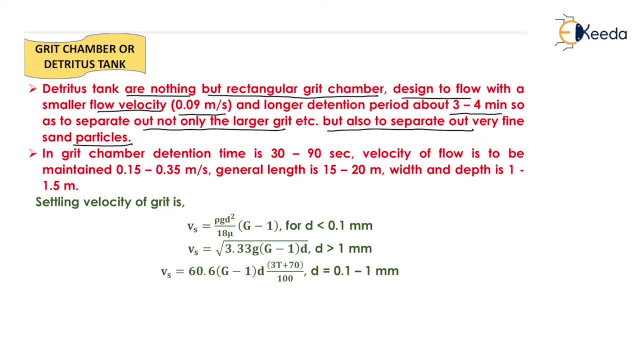 and provided with longer detention time. clear now. in grit chamber the detention time is 30 to 90 second, but in detritus tank the detention time is three to four minutes. velocity of flow is 0.15 to 0.35 meter per second, generally kept as 0.25 meter per second. but 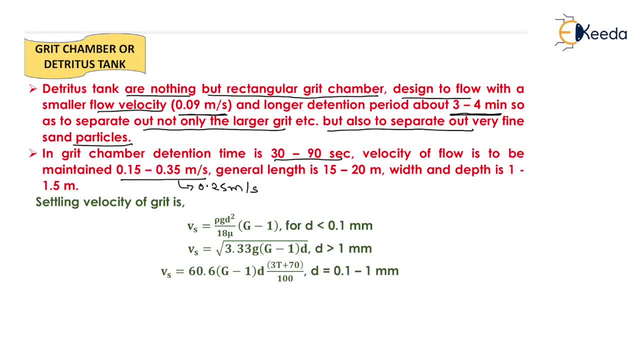 in detritus tank, the velocity generally kept as 0.09 meter per second. now the general length of both the tanks are same, that is 15 to 20 meter. width and depth is also same, that is 1.5 meter. now if we want to calculate the length of both the tanks, we have to calculate the length of the tanks. 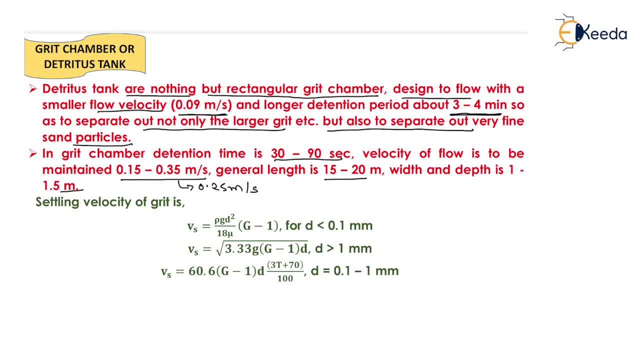 that is 15 to 20 meter. width and depth is also same. that is 1.5 meter. width and depth is also same. we can also calculate the settling velocity of the particles, or grit that. it can be computed by the stokes law that will be known as rho. g d square upon 18 mu into g minus 1. okay, we had already used. 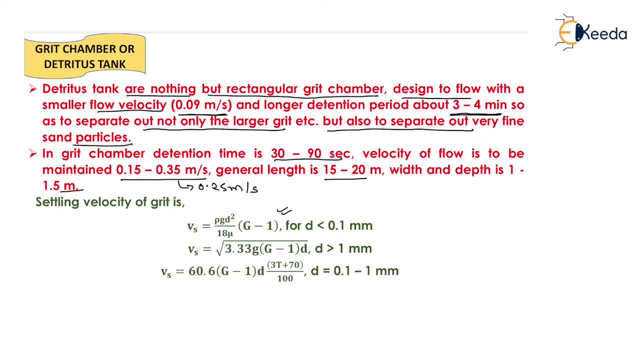 that formula in the sedimentation tank of water treatment unit. here also the formula is same, that is, rho g d square upon 18 mu into g minus 1 for diameter less than 0.1. this is known as stokes law. clear now. the another formula for the stokes law is the stokes law and it is known as stokes law. 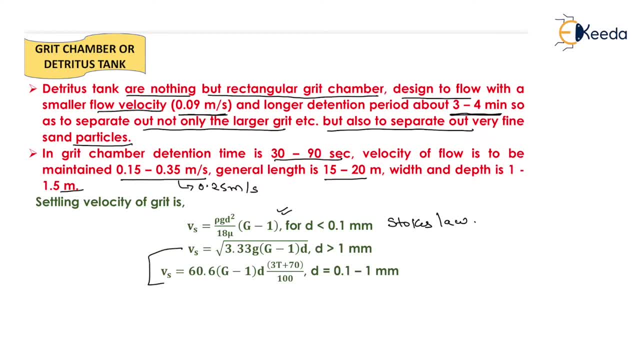 which will be used rarely is the last two formulas, that is, Newton's law when particle is greater than 1 mm, and the last one is Hazen's modified equation, Hazen's modified equation, but these two formulas will be used very rarely. only the Stokes law will be used mostly. okay, now, skimming tank will be there, that is. 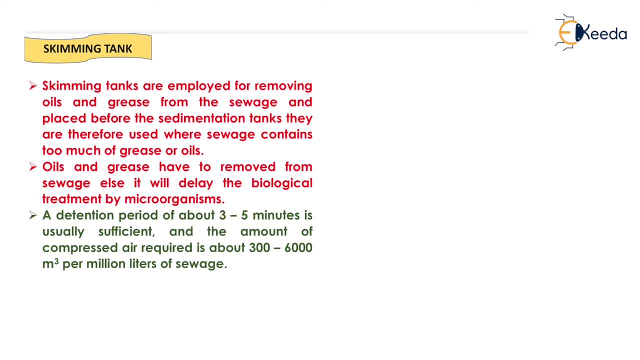 the next unit. now why we used to skimming tank in the treatment process? because to remove the oil and grease from the sewage. that's why they are placed before the sedimentation tank. therefore, when sewage contains too much of grease or oil, we generally need sediment. sorry, skimming tank. okay now. 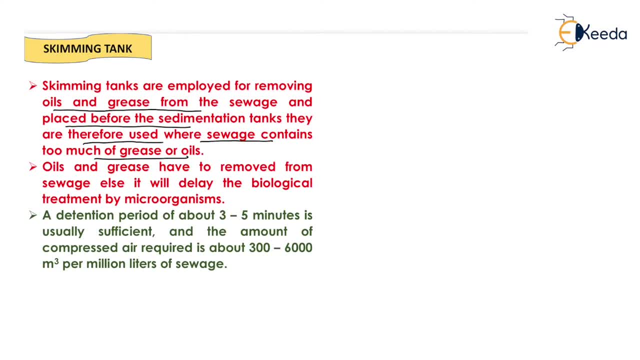 skimming tanks are employed for removing oil and grease from the sewage and placed before the sedimentation tank. they are therefore used where sewage contains too much of grease or oils. it means that when sewage contains too much of oil and grease, we need to provide the skimming tank for the removal of oil and grease. now, oil and grease have to be. 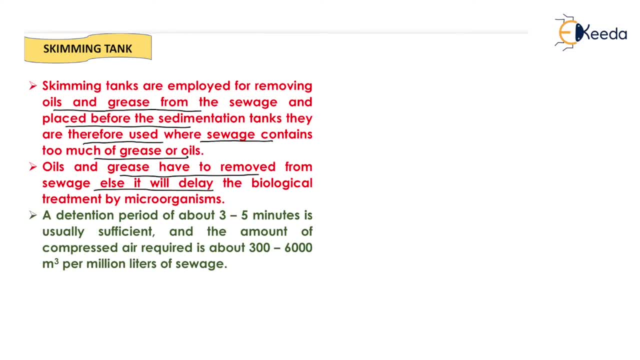 removed from the sewage, else it will delay the biological treatment by microorganism. if we don't remove the oil and grease, then the biological treatment will be delayed. okay now, a detention period of about three to five minute is usually sufficient, and the amount of compressed air required is about 300 to 6000 meter cube per million. 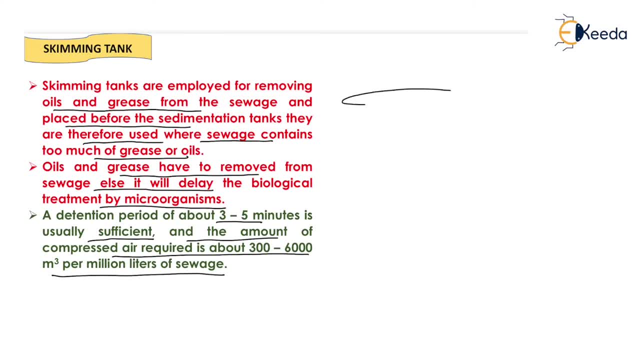 liter of sewage. suppose that we have a large container here containing wastewater from the sewers. okay, now that water will contain oil and grease at the top, like this, and remaining water will be like this. now, at the bottom, there will be some holes, which is generally provided, or? 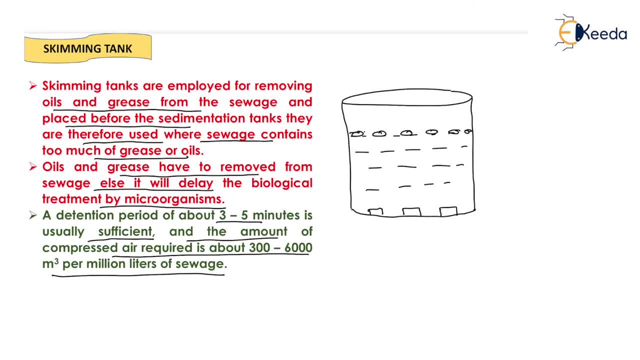 there will be some equipment which is generally provided for sending the compressed air. for sending the compressed air, now, at the top, there will be a skimmer like this. there will be a skimmer like this having cups at regular interval, and it will connect with a channel like this which will dispose. 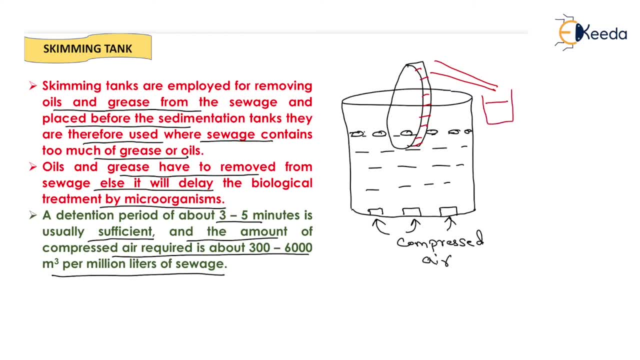 all the oil and remove in a oil and grease in a container. okay, now, when this skimmer will revolve like this, we will supply compressed air from bottom. now this compressed air will take all the grease and oil particle to the surface and from the surface it will become into this cups and from this cups it will. 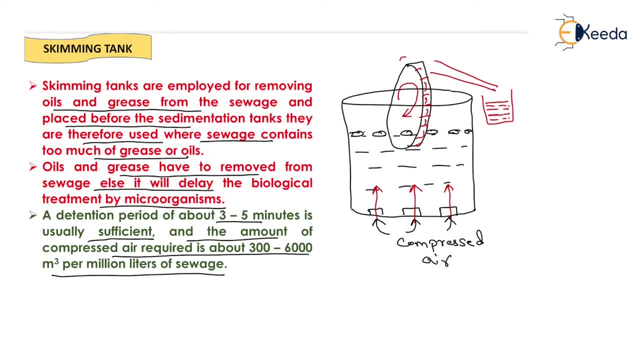 come to that topmost point and during the downward journey of skimmer, all the oil and grease will come into that channel and from that channel it will be stored in a particular container which is kept outside that large container. okay now, in this way we had removed the oil and grease from the sewage water. 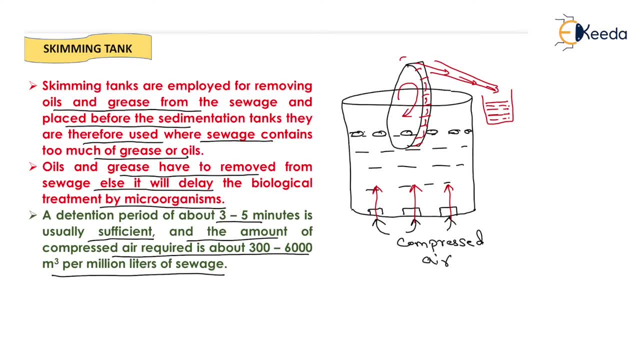 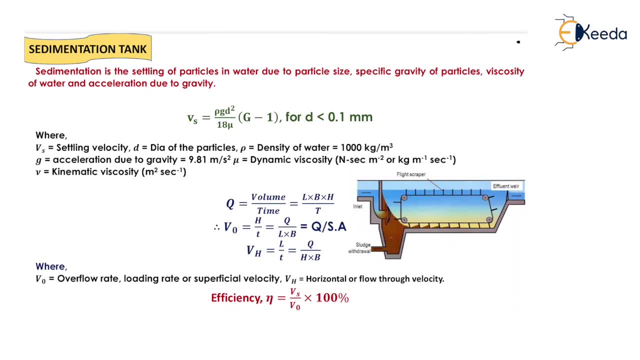 clear now. that is the skimming tank. now we can move to the next process, that is, sedimentation tank. we had already discussed the sedimentation tank in the water treatment unit, and the same sedimentation tank will be used in the wastewater treatment also. now the sedimentation is the settling of. 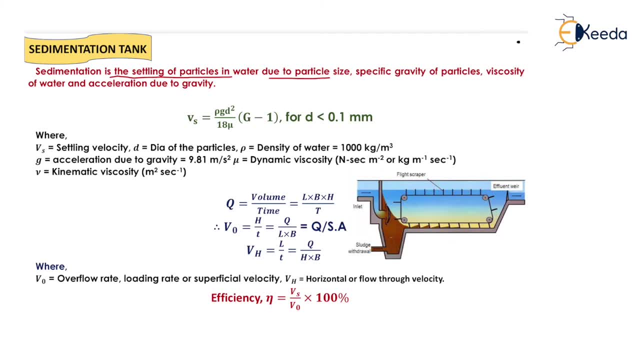 particles in water due to particle size, specific gravity of particles, viscosity of water and acceleration due to gravity of settling velocity. we had already discussed that stocks law is used for the calculation of settling velocity and it will be equals to rho. G d square upon a 10 mu into G minus one for diameter less than 0.2, 1. now we all. 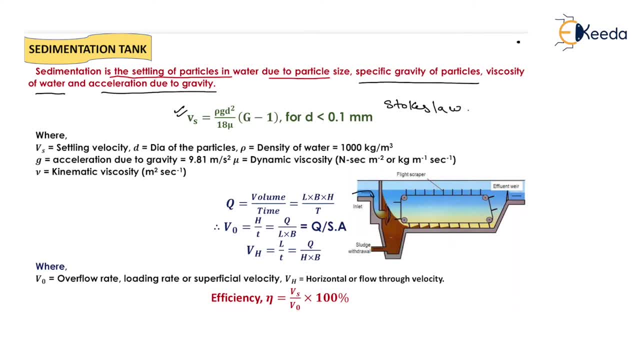 know that, what is overflow velocity, or loading rate, and what is horizontal flow velocity, or flow through velocity. okay, we had already discussed this topic in detail in the water treatment unit, so we will directly use the formula to. that is, VH will be equals to L by T and it will be equals to discharge upon length into. 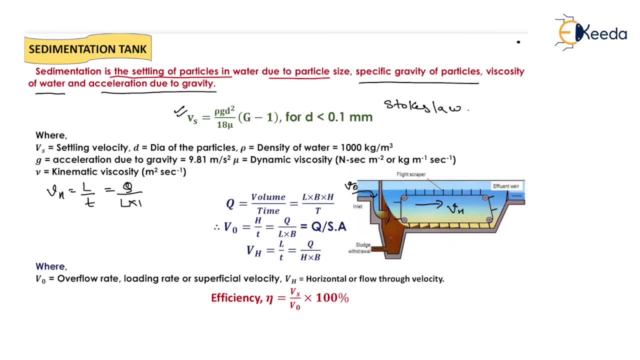 or it will be equals to discharge upon height into width. clear Now. similarly, V naught will be equals to H upon T, which will be equals to discharge upon L into B, which will be also known as discharge upon surface area. One more formula will be there, that is the efficiency formula. it 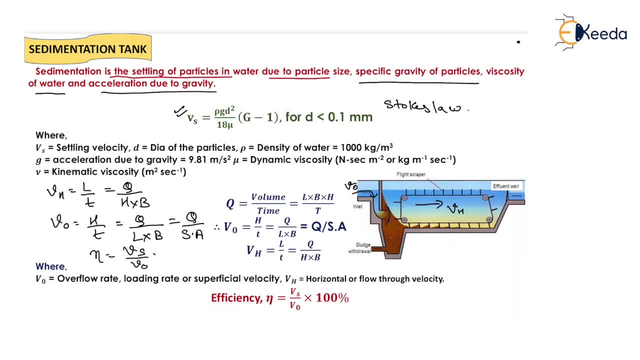 will be equals to the output upon input into 100, that is, VS upon V naught into 100. So we had shown all this formula that is length into width, into height, upon time. Similarly, V naught will be equals to discharge upon surface area, VH will be equals to discharge upon B into H and efficiency. 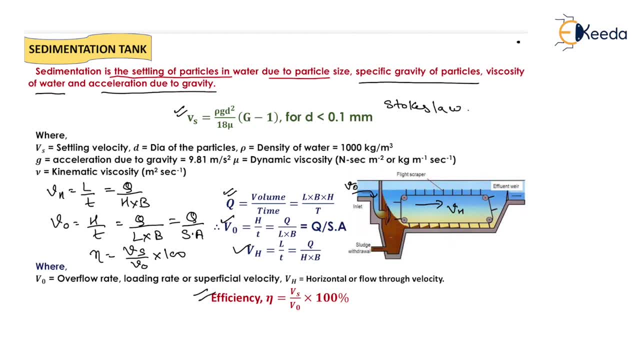 will be equals to VS upon V naught into 100.. That will be all about the preliminary treatment of wastewater. Thank you very much, students.